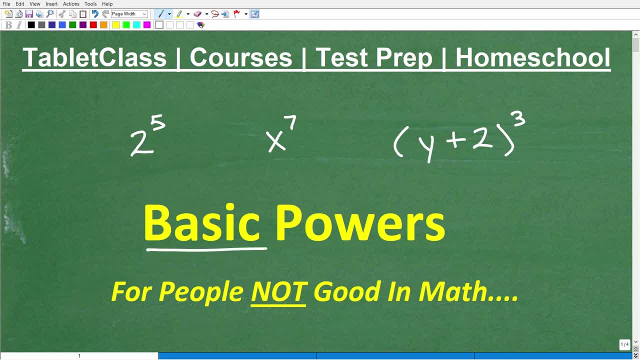 Okay, let's talk about basic powers or just powers in mathematics, And you can see down here I have for people that are not good in math. So if this caught your eye and you said, Oh yeah, I'm definitely not good at math And I'm glad that you found me because we need to get rid of this, All right, everyone can be great in math. However, what you need to do is find somebody that can really you know, teach you in a way you like and understand, And that's going to be my goal for this video. So we're going to talk about basic powers, or talk about the parts of a power, And 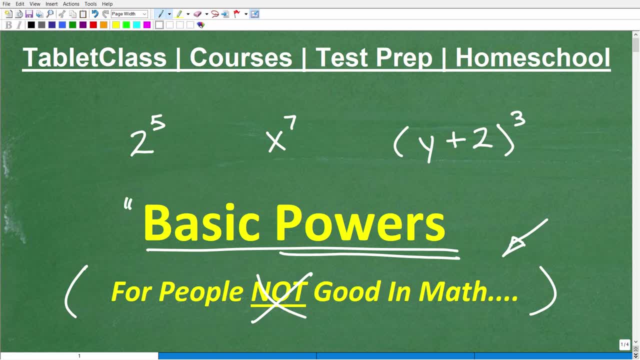 how to kind of, like you know, work with them in a basic level. Okay, and when you study things like algebra, powers and exponents are very, very important, So you definitely need to understand that And it's not that difficult. So we're going to start from the very beginning and kind of build your knowledge up a bit here. So by the time you leave this video, you're going to have a basic understanding of powers. But before we do that, let me go ahead and quickly introduce myself. My name is john. I'm the founder of tablet class math. I'm also a middle and high school math teacher, And 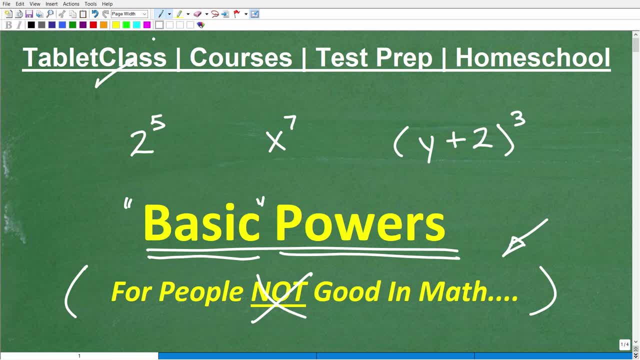 over several years, I've constructed what I'd like to believe is one of the best online math help programs there is. of course, I'll let you be the judge of that. you can check out my math help program and following the link in the description of this video. But what you're going to find when, when you get to my site, is 100 plus courses ranging from pre algebra, algebra, geometry algebra to pre calculus and a ton of test prep courses. So if you're studying for a GDSAT, ACT, maybe a teacher certification exam, ton of other type of exams- I can help you out And I also do a lot with. 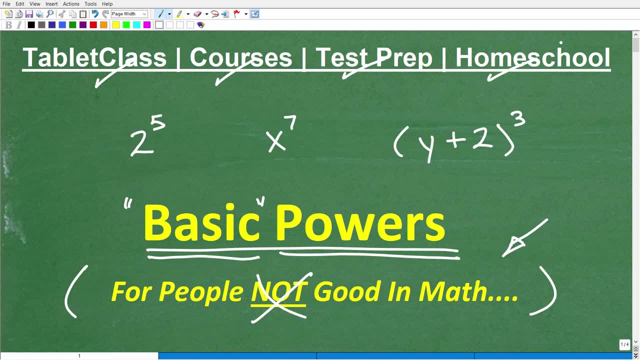 homeschooling. Now, one thing you do have to do to be great in math is to take great math notes. So if your notes aren't kind of where they need to be, you need to improve your note taking And you can use my notes in the meantime to study from. So I'm going to leave links to all this stuff in the description of this video. All right, let's get into this. basic powers. Okay, for people who are not good at math, we could just dispel that. Okay, everyone could be great in math, But let's talk about powers, All right. So when I use that word, 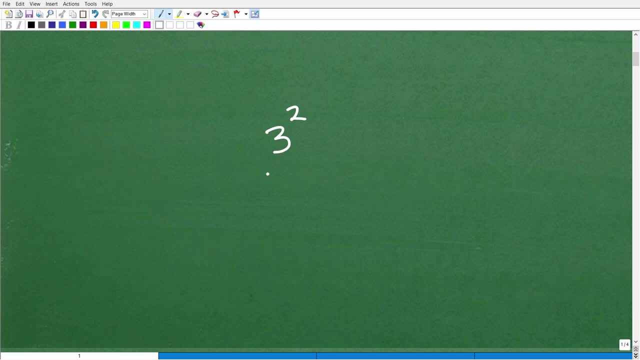 powers. what am I talking about? Well, I'm referring to something like this: Okay, now, how would we, you know, say this or describe this: this would be three to the second power, right? So that's how you would, you know, most people would be okay with you know, describing this as three to the second power, or three squared, okay, which is perfectly fine. What about this? this would be three to the third power, or three cubed, And then we have three to the fifth power. 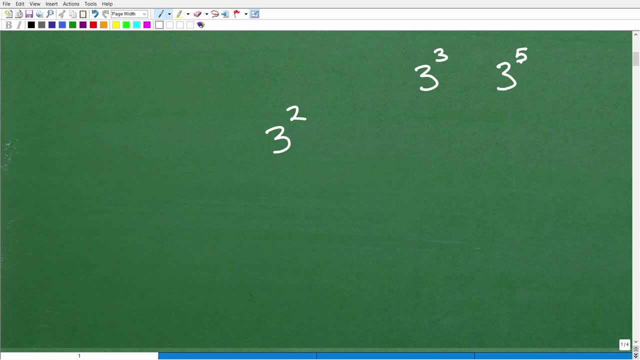 then we're like: well, three, you know we don't have like a squared or cubed, we kind of do, but nobody kind of says that. So this whole thing right here is considered a power Okay. so when we're talking about powers, we're really describing this whole entity, Okay. but there's 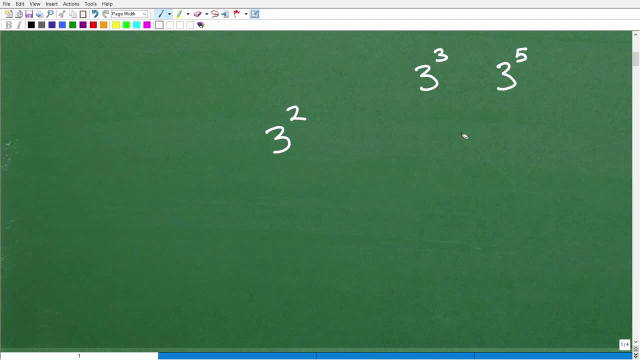 some parts here to it. Okay, And what are the parts? Well, there's this big number down here, this three. we call this guy here the base And this little number up here we call the exponent. Okay, so base and exponent, the whole thing together is a power. But what is this really? 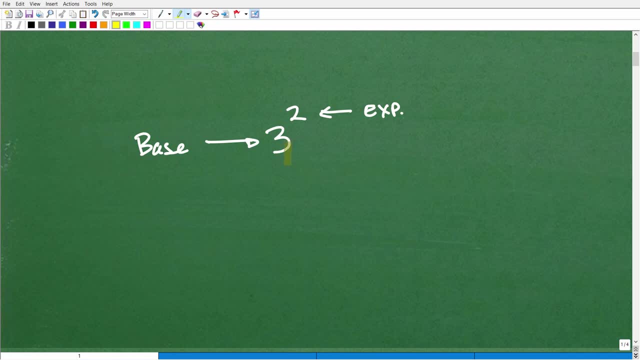 saying to us: Well, effectively, powers are just kind of a shortcut way of writing something that's being multiplied by itself multiple times. So this three squared is saying: take the number three and multiply it by itself two times. So that would look like what? three times three. Okay. 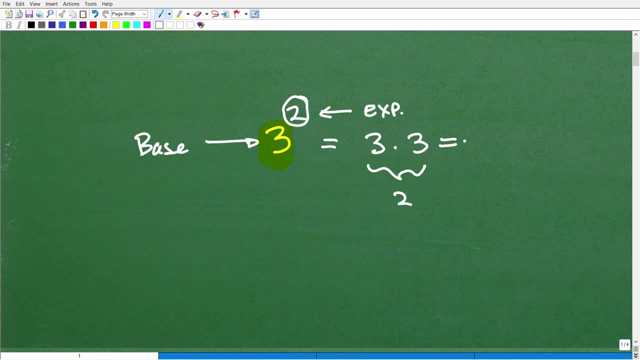 so here is the two times. So three times three is of course equal to nine. So three squared is equal to nine. Of course that's the same thing as three times three. Okay, let's do another quick example Now. if this is very basic for you, well, that's good. That shows me that you 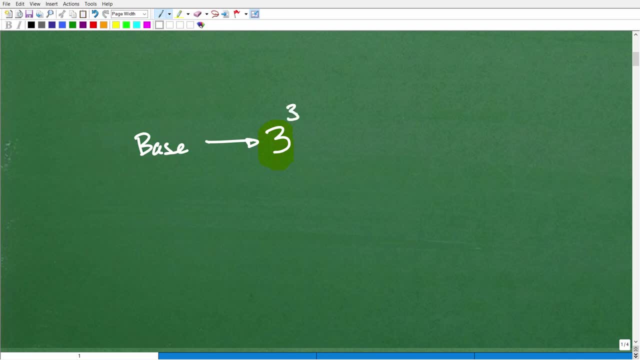 obviously you know, have some understanding of this stuff, But let's go ahead and do this. This is what three cubed, And that means take three and multiply by itself. three, three times three times three times three. Of course, that's going to be nine times three, or 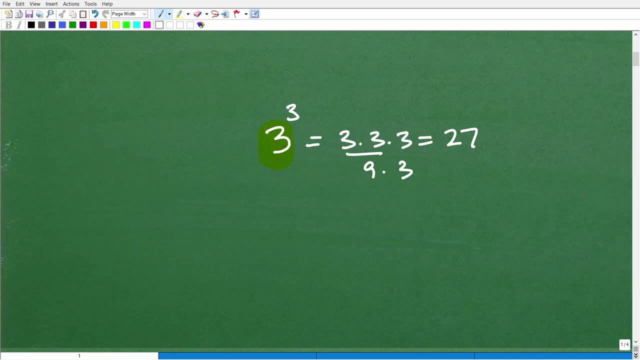 27.. Okay, so that's how you know the essence of powers works. But let's just get some definitions down Again. the big number down here is called the base, Okay, and that small little number is called the exponent. But this also this base and exponent and power concept works with things. 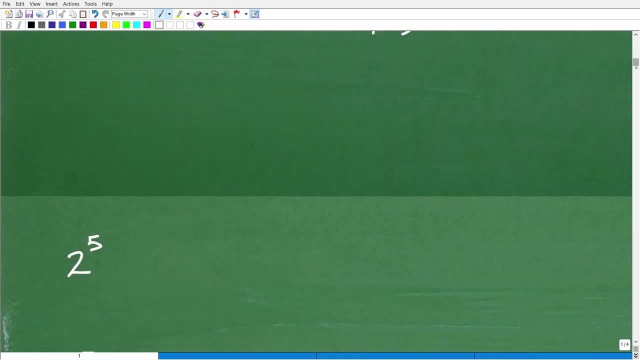 outside of just numbers. Okay, you can do all kinds of stuff with power, So let's go ahead and just review Here. I have two to the fifth, Okay. so this is in power form, right here. Okay, we could see our base is two, the big number and our exponent is five. So one thing. 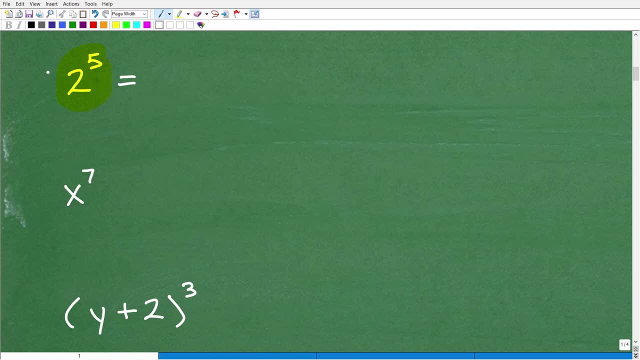 we're working with powers and exponents. sometimes we like to write a power in what we call expanded form. Okay, now, what would that be? Well, it would be two times two. we're going to take two and multiply it by itself five times. So two times two, times two. okay, times two. 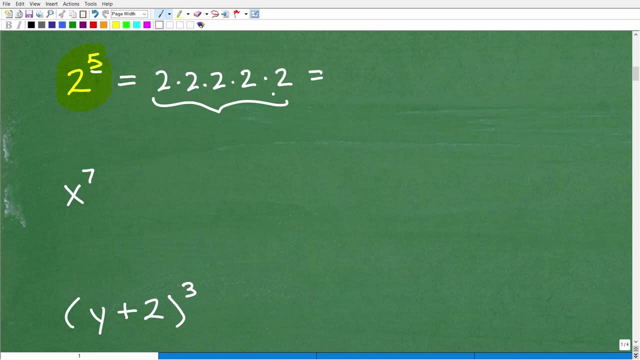 you can see if I'm taking two and multiplying by itself five times. I don't want to, like you know, write this. Imagine if this 50, whether it's like two to the 50 power, you'd have to write a bunch. 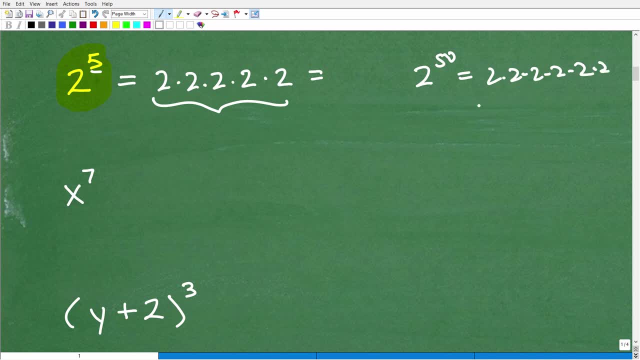 of twos. you know your hand would fall off. you know you wouldn't have enough paper or enough time to express this. So that's why we have powers. It's a shortcut way of writing things that are being multiplied over and over and over again. by itself, Okay, But here we could calculate. 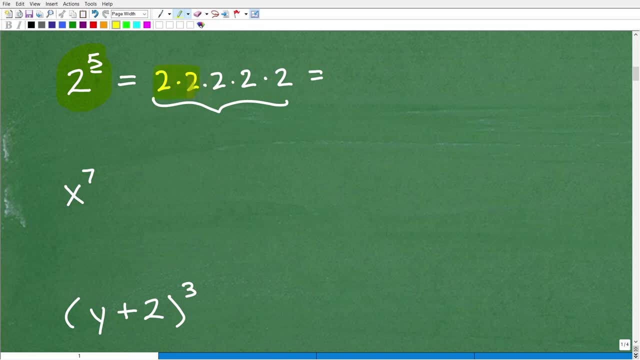 this, Hopefully without the aid of a calculator. we got: two times two is four. Okay, so that's four times two. This gives me an eight, and eight times two is 16.. 16 times two is 32.. Okay, so two to the fifth power is 32.. Now, if you want to, 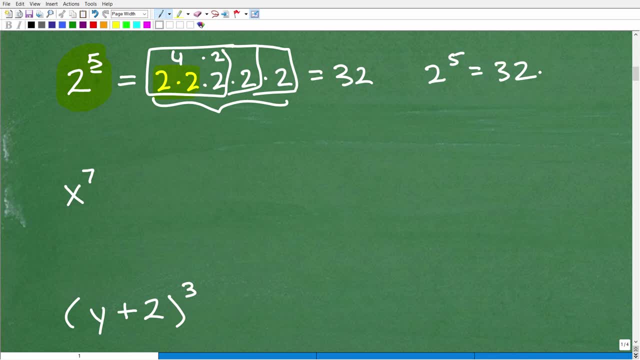 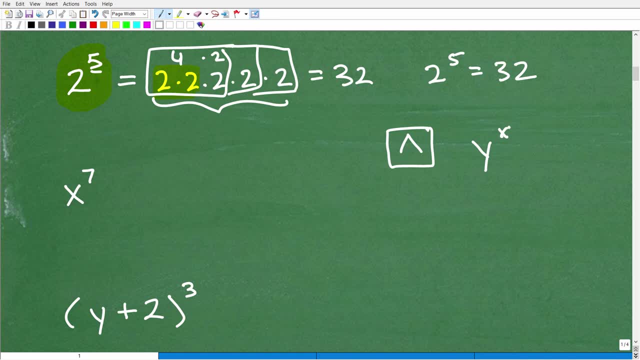 It's going to be this little button that's called a carrot or something like this: Okay, y to the x or x to the y, These are probably the most common buttons. So you want to get used to being able to calculate powers on your calculator. So, for example, two to the fifth power you can go in. 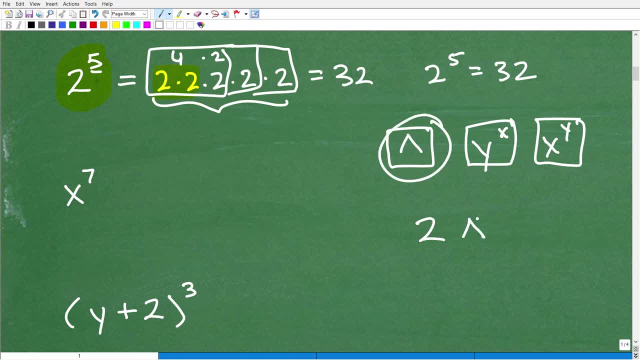 and go two. You probably would use this button. Okay, this is a very common button. It's called a carrot Two to the fifth power. You should look at your calculator. that the one you're going to be using. if you're already a student, You should look at your calculator. that the one you're going. 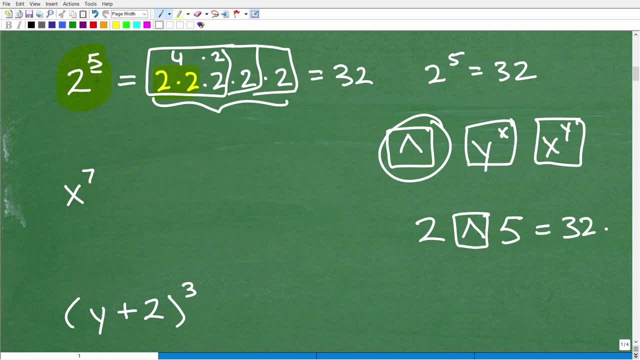 to be using if you're already a student, and play around with it just to make sure you can actually get the right answer. Okay, so if you don't have this button, look for one of these and then just kind of play around with it, Make sure you can actually calculate or compute a power. 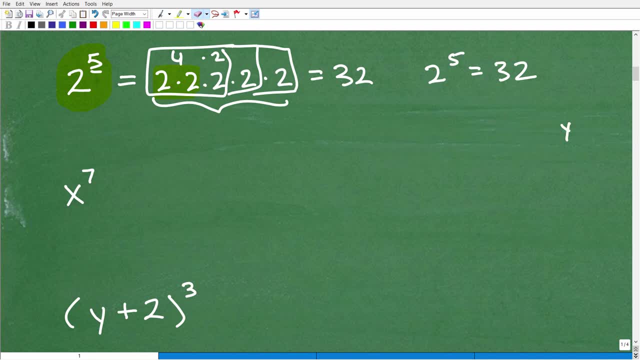 on your calculator. Okay, let's talk about this guy right here. X to the seventh power. So what is the base? The base is x and our exponent is seven. But what does this mean? Well, it means multiply x by itself seven times. 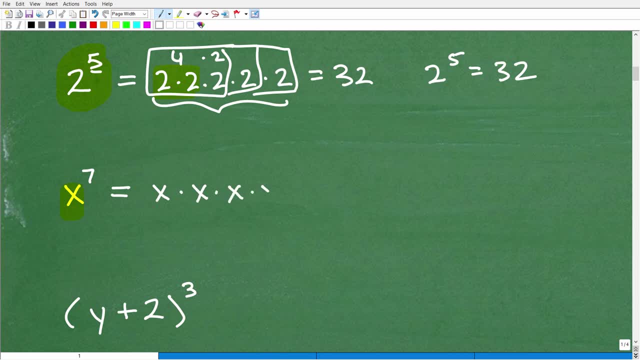 So this is x times x times x. There's three, There's four, There's five, There's six, There's seven. One, two, three, four, five, six, seven. This is x to the seventh in expanded form. Okay. 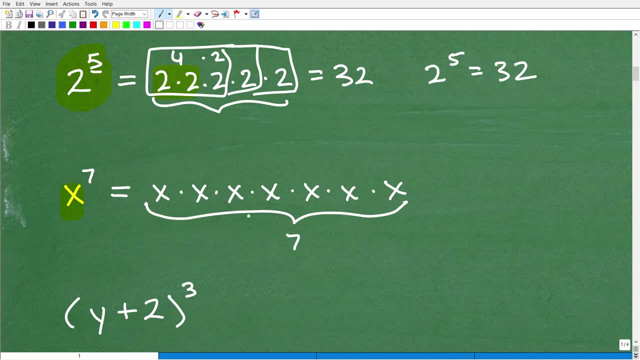 now, why do we want to, you know, go from a power to expanded form? Well, let's look at, let's say, you had x to the seventh over x to the fifth. Okay, so let's say we're trying to figure this out. Then there's rules for this. But you know, for just the fact. 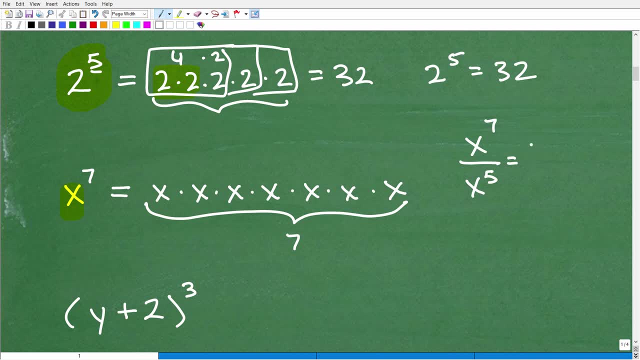 that you know this. you could figure this out right now. So x to the seventh, that means there's seven x's up here: One, two, three, four, five, six, seven over. x to the fifth is how many x's? 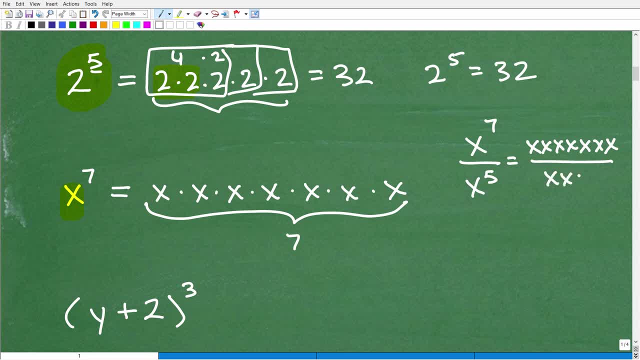 down in the denominator. Well, there would be five, One, two, three, four, five, And this is all multiplication. So these are factors. So five of these x's could take out five of those x's up there. We can just cross cancel. 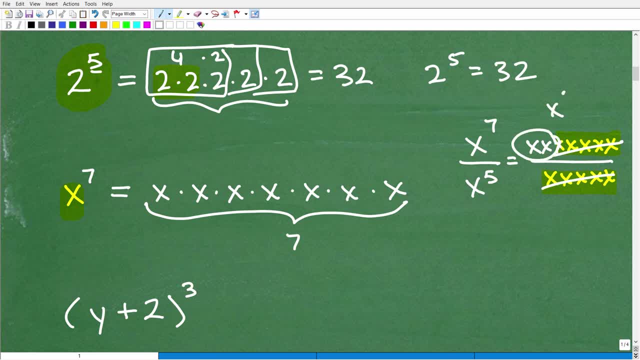 These guys right there And I'm left with x squared. Okay, so x to the seventh over x to the fifth is in fact x squared. So just a little bit. you know I'm kind of sharing a little bit more here, But you know, you can see that this is not complicated stuff And it's very, very. 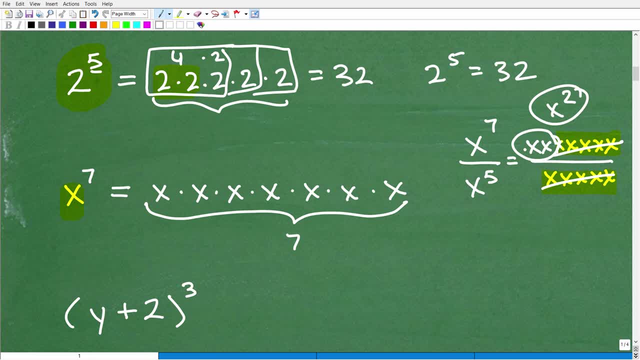 important because in algebra and mathematics you're dealing with a lot of things that have powers and exponents. You got to know how to work with them. But again, we're just going to start building up your knowledge one step at a time. 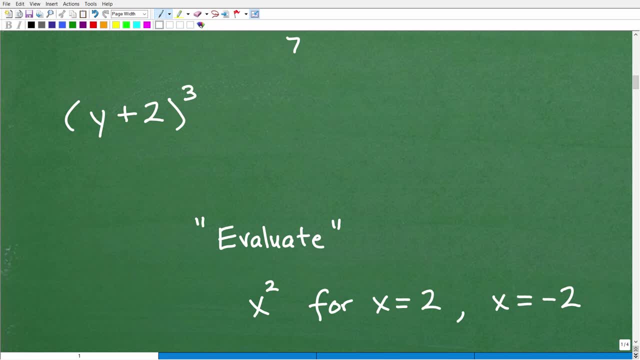 So let's take a look at this expression right here: Y plus two is three. So you're like, oh man, what? what's the base? What's the exponent? Well, this whole thing right here is considered the base. Okay, this is the base, And it's saying: hey, multiply y plus two by itself three times. 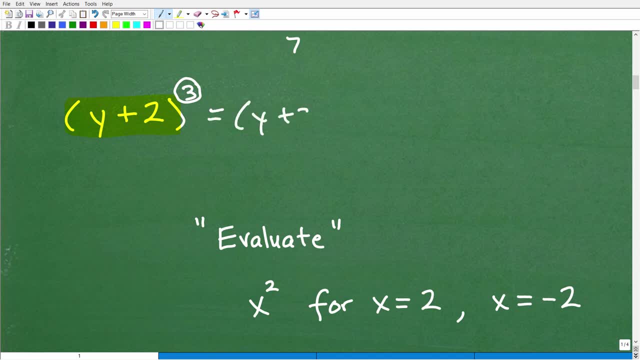 So would this would be equivalent to y plus two. You guessed it: Y plus two times a y plus two. All right, so this is typically called expanded form, And then we have our form base exponent. We don't have to make it any more complicated than that. Now, one thing I do: 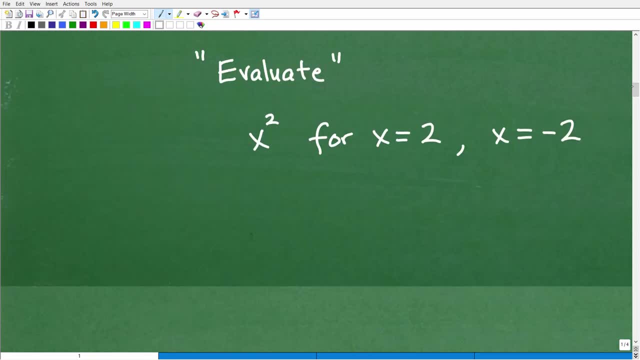 want to talk about real quick, before we wrap up this basic video, is this word: evaluate. Okay, typically in math you see this. especially in algebra you'll get problems like evaluate- this expression- I'm going to use x squared for a particular number. Now what it means, this word. 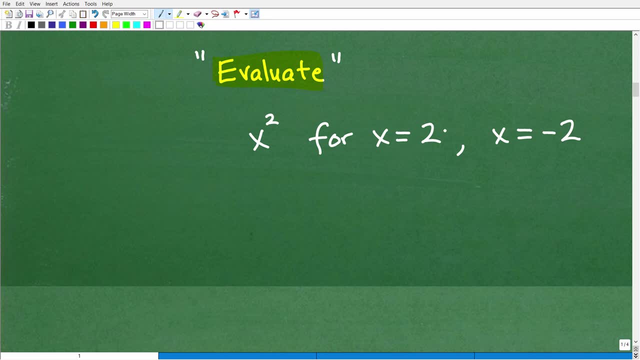 evaluate means take the number. okay, for example, x is equal to two. I got two prompts here we're going to look at both. take this number, replace this x right there with this number, because x- we're saying x- is the same thing as two, So replace that x with. 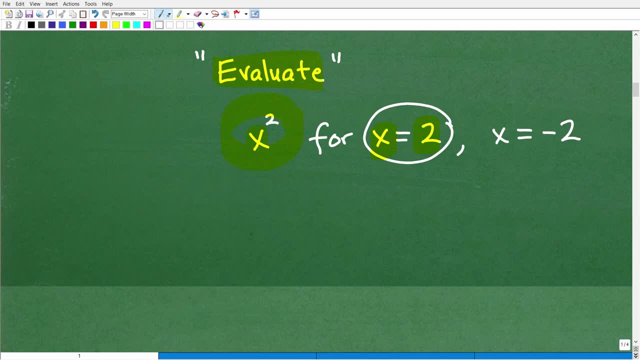 that two and then figure this out. So here is what I want you to remember. I really want you to take a big mental note. here is: anytime you're evaluating or plugging in numbers for variables in an expression in algebra, always use parentheses. Okay, always, always use parentheses. you cannot. 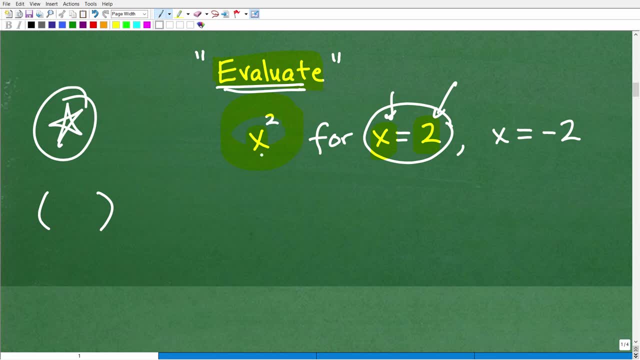 be wrong. So let's go ahead and do this here. So x squared. let's evaluate x squared, for x equals two. So I'm going to use parentheses to replace this x. I'm going to plug in two for this x, because we're saying x is equal to two squared. So now I'm going to figure out what two squared is. 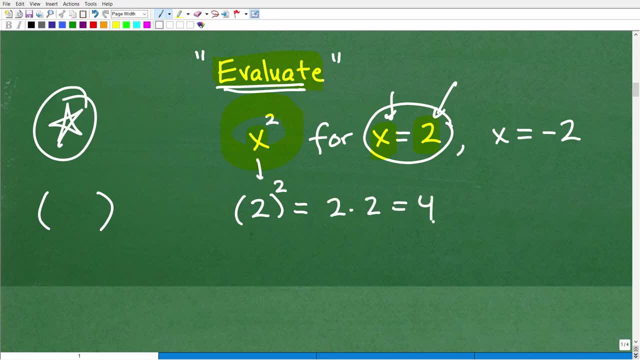 of course, that's two times two And that's equal to four, All right, So you know, if you're understanding that, that's excellent. Okay, matter of fact, let's give you a nice little happy face So you can feel great about yourself, All right, And you're like: 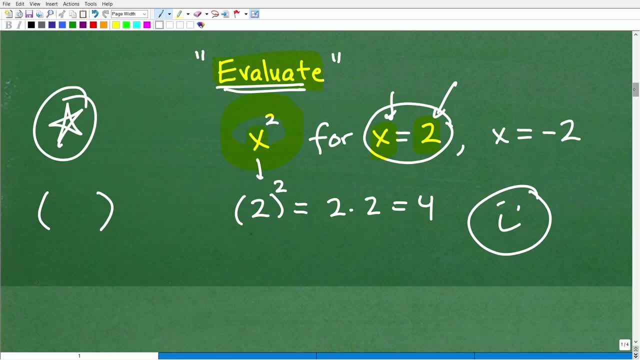 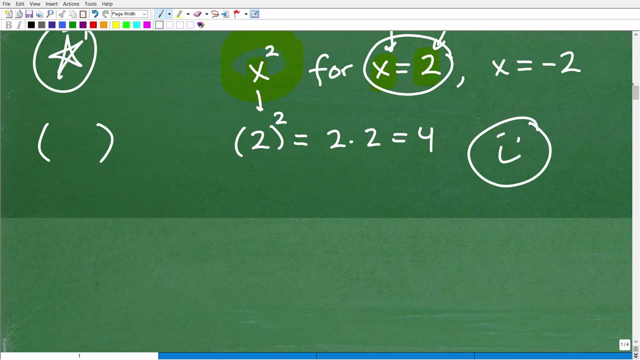 I'm learning this stuff, You're good. Yeah, absolutely Right. You know we don't need to be having these mental, negative mental thoughts like I'm terrible in math and stuff. The first thing, if you're trying to learn math, the first thing you need to do is get rid of any. 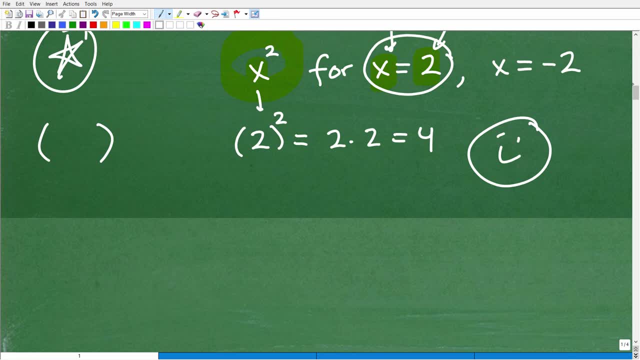 negative thinking. Okay, you just need to find someone that could teach you and be, you know, committed to learning this stuff. All right, let's take a look at this. one: x squared. let's evaluate x squared, for x equals negative. two: 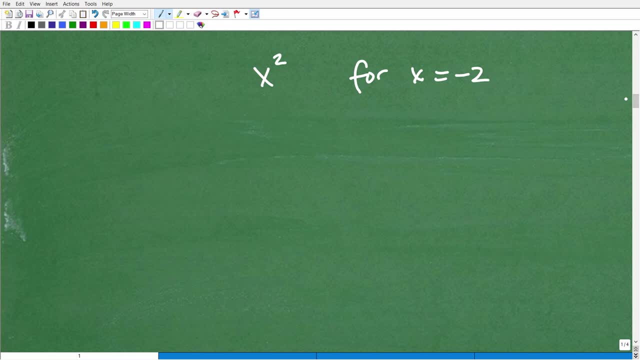 Now this gets a lot of students in trouble, Because if you don't use the parentheses, students would go: okay, negative, two squared, And the answer is either going to be negative four or four. All right, So if you're familiar with positive, negative numbers, you know which one. 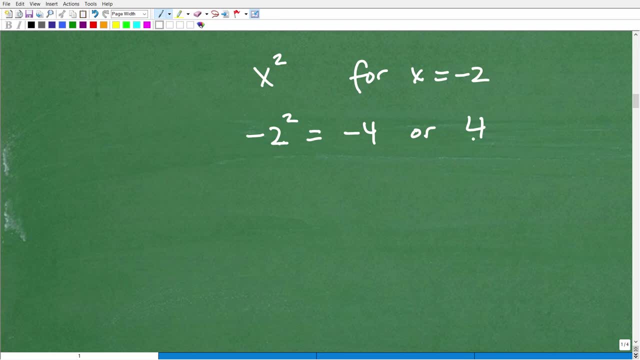 is, it is going to be negative four or four. So maybe you want to kind of think about that for a second. But if you are using my advice when I said to use parentheses, you're going to stay out. figure out what x squared is, for x is equal to negative two, So x squared. I'm plugging in the 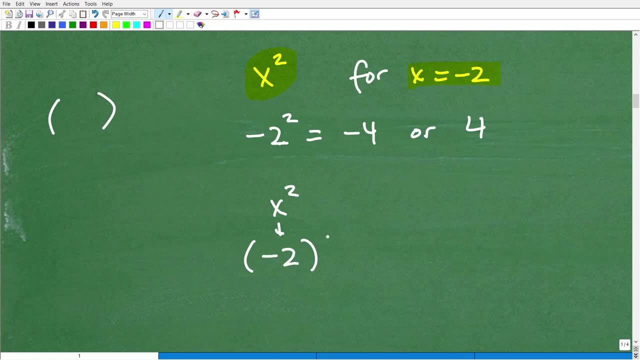 value for x. with parentheses, that's going to be negative two squared. So now, when you see it this way, this is much clearer to say: Oh, okay, I need to take negative two and multiply by itself twice. Okay, two times. So that's negative two times negative two And negative times a negative. 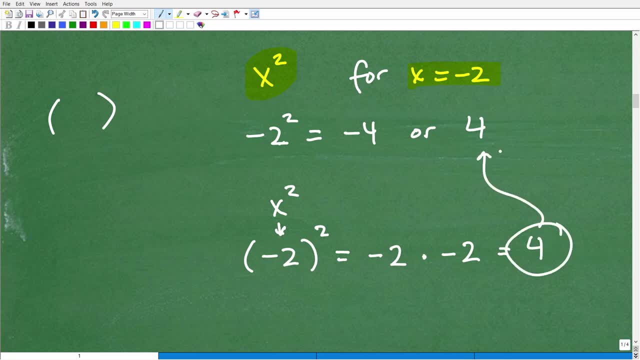 is a positive, So we have positive four. this is the correct answer. Now, if you knew that, then I must give you a big smiley face with the good old fashioned 1984 Mohawk with extra aquanet hairspray. Okay, yes, people actually walked around like that. 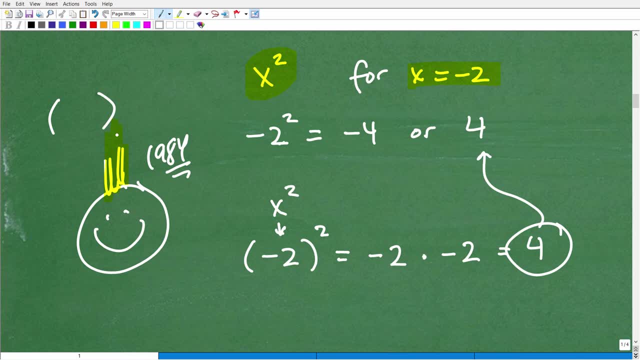 Way back in the 80s We thought we were cool. But you know, I guess you know that wasn't that cool. because that fads not around. probably a good thing, because you know that much hairspray in. 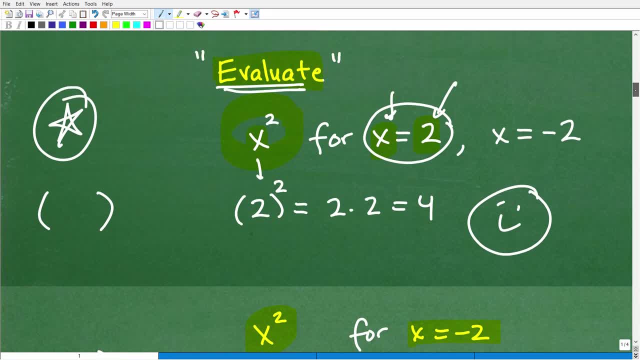 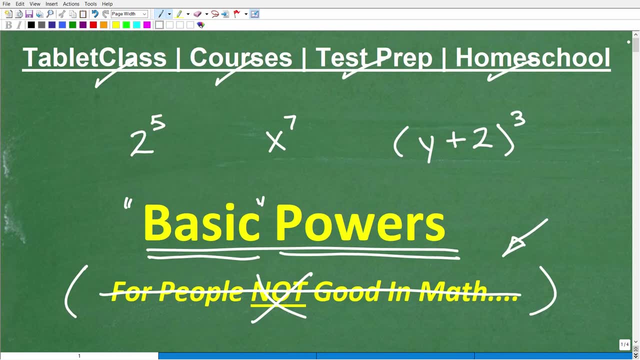 your hair is probably not a good idea, Anyways. so if you understand everything I covered right here in terms of powers and exponents, you're certainly on your way to learning more about powers and exponents. And there is more: you need to know how to deal with multiplication of powers and exponents division, you kind of 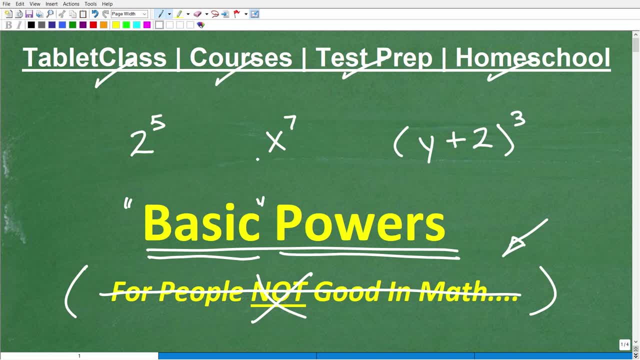 looked a little bit. example there and other things, Okay, but you know again. all right, mathematics is a journey And you have to. it's like a staircase, right? You're not going to get up here on the top of the stairs by just magically jumping up here. Maybe if you had that power.